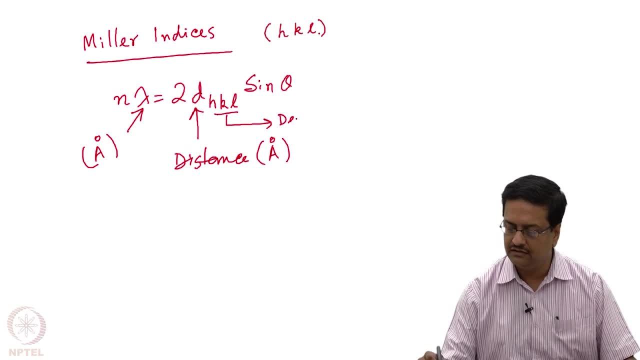 indicate the planes. So it is the designation of planes. So when we are talking about a set of parallel planes, sorry, sure, So this is the designers label of a plane of a particular degree. So if we say: so it is a nickname of hieroglyphs for any plane in Honeys 백sl, and it is 67 review values, 742 SUV. so of course, Diouf. and how stronger and stronger it is for any plane in Hellen Purple. 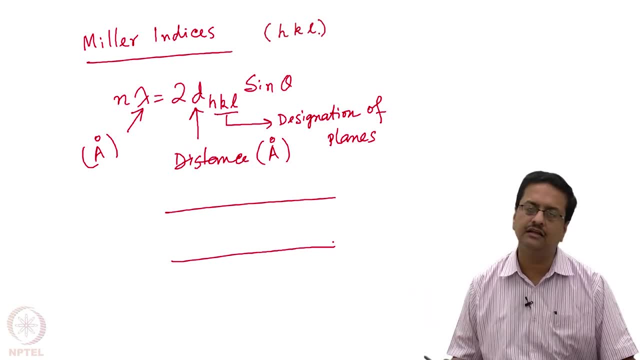 then we therefore know from this set of parallel planes there are видим to detective numbers of cheesy curve, So as aals, the data forTaI macro expressions are strong. So Suppose these are two set of parallel planes in a crystal lattice, the distance between 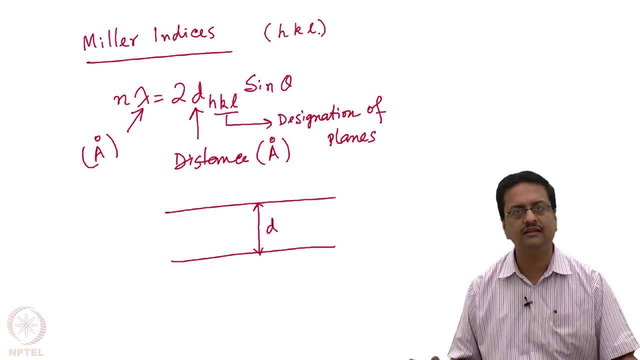 these two parallel planes are called as d, and we designate these planes as h, k and l. as a result, we identify this distance as d, h k, l. So to do that, we need to know how to designate these h k ls, what are the possible values of h k ls, and then we should know the. 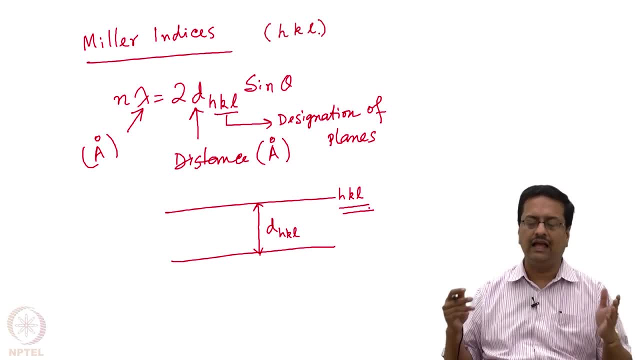 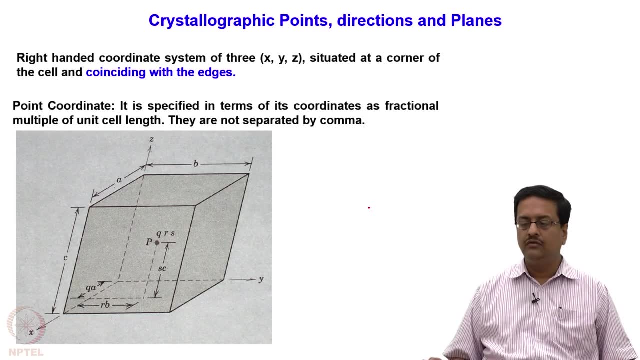 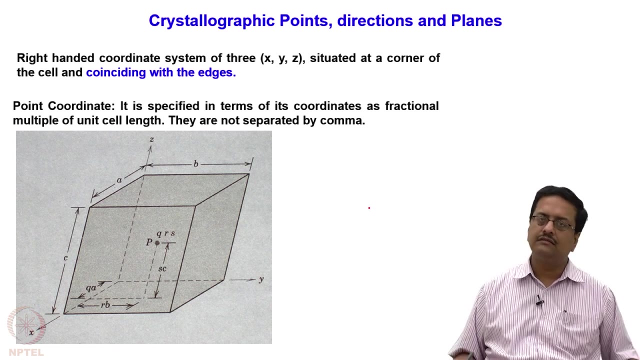 significance of those planes with respect to the axis x, y and z. So to know about that, we need to know about the crystallographic points, directions and planes. So in this circumstances, in the crystallography, in while considering a lattice, we always use a right handed coordinate. 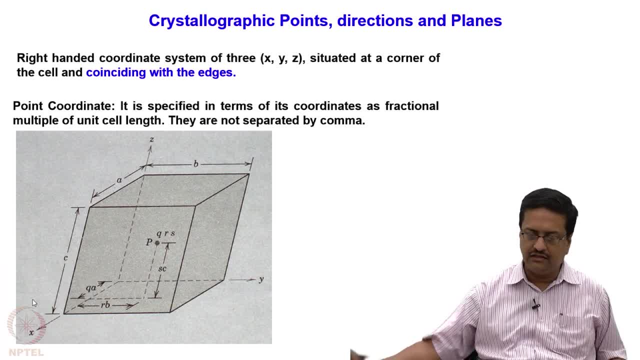 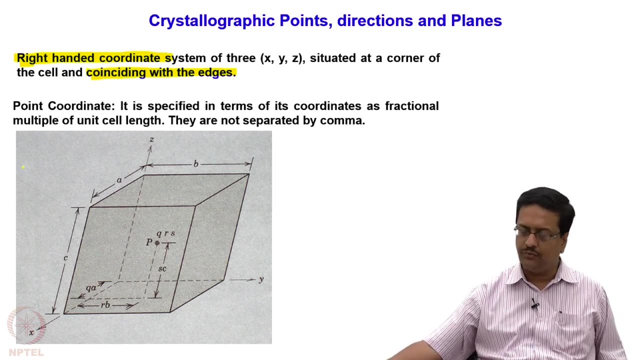 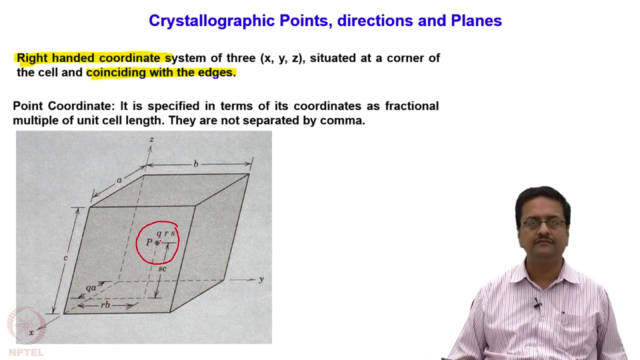 system, as is indicated here, the right handed coordinate system of three axis: x, y, z, and with the coinciding with the edges. So now, if we have a point inside a lattice which is designated here as P, then what should be the coordinate q r s of that point P? This point q r s has the 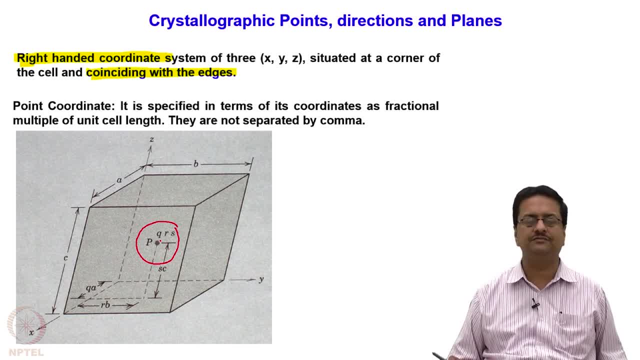 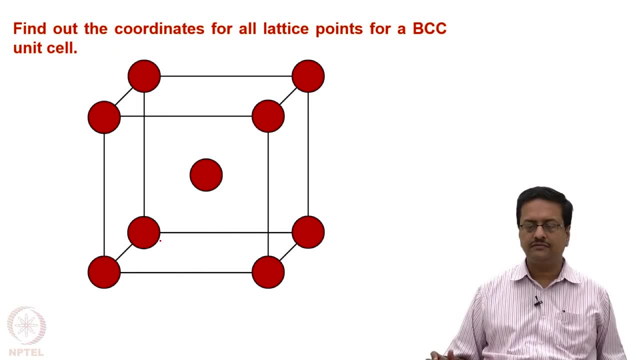 coordinates, which are the fractional coordinates with respect to the unit cell parameters a, b and c. So, in case of a body centered lattice, we have atoms at the 8 corners. as you can see, the atoms at 8 corners and the atom at the center of the 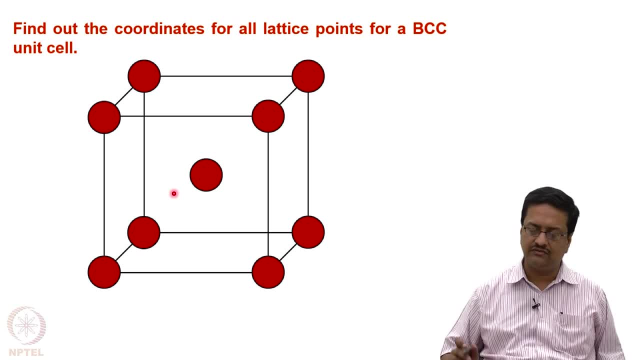 lattice. What are the coordinates of those corners with respect to a given origin, which is 0 0, 0? The ones which are 1 unit along x, 1 unit along y and 1 unit along z are designated as 1, 0, 0, 0, 1, 0 and 0, 0: 1. set of coordinates, set of points, because those are at 1 unit. 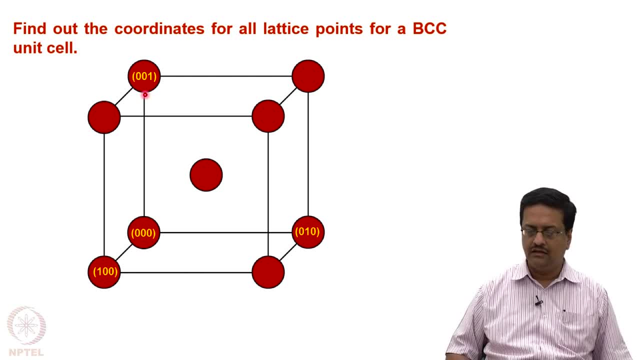 away from the origin. Then the other corners which are now here: 1, 2 and 3,. 1, 0 and 2 and 2, these arezing a whole set of coordinate lines, Because those yang 1 unit away from the origin, Then the other corners which are now here: 1, 2 and 3,. 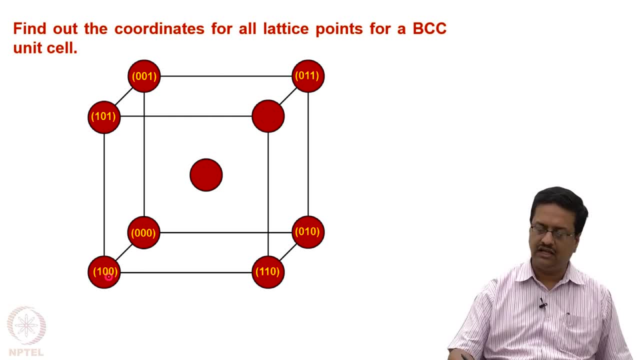 they are first one unit away along x, one unit above along z and 0 along y. So this point is 1 0: 1.. Similarly, from here you go one unit along y, you go one unit along z and not going anything. 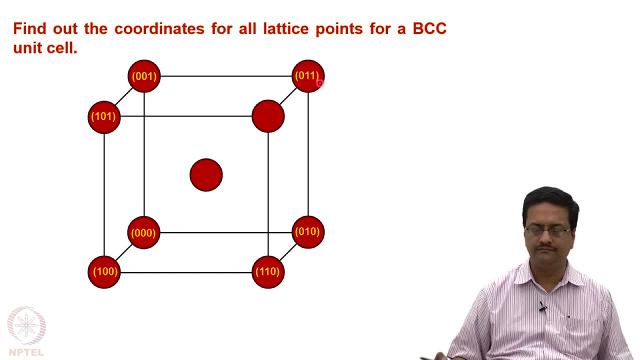 anywhere along x means it is 0: 1, 1.. So like that, the opposite corner of origin becomes 1: 1, 1.. We travel one along x, one along y and one along z, so it becomes 1: 1, 1.. The point at the center of the lattice, which is a body centered unit, shell. 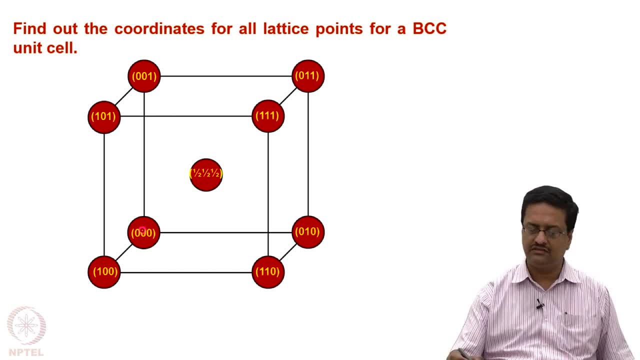 then is half half half. that means Z x, 1 plus 1. You from the origin. we travelled half along x, half along y, and then gone halfway along z and reached the center of the lattice and designated it as half and half half half. So for your homework, 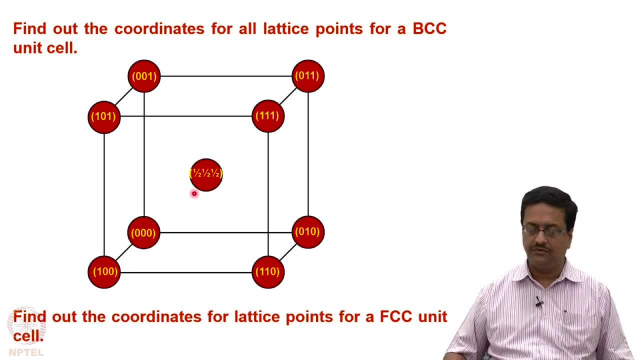 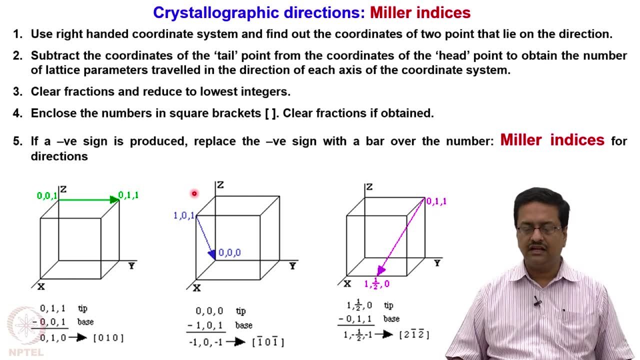 you find out the coordinates for lattice points for the FCC unit cell. So now let us try to identify the crystallographic directions and the corresponding Miller indices. for that, Once again, we use the light handed coordinate system to find out the coordinates of the two points that lie on. 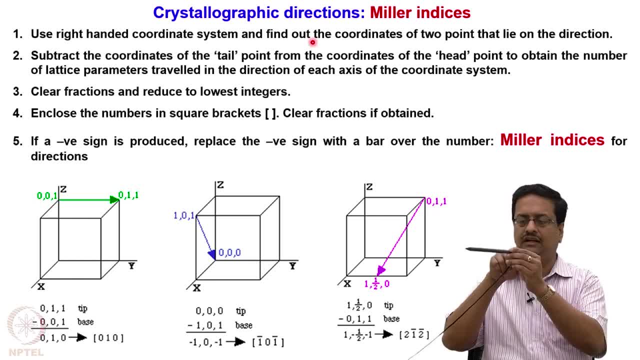 the direction. Suppose, if this is the direction, I want to find out the two points, the bottom point and the top point, and determine the corresponding coordinates. Then you subtract the coordinates of the tail point From the coordinates of the head point to obtain the number of lattice parameters travelled in the 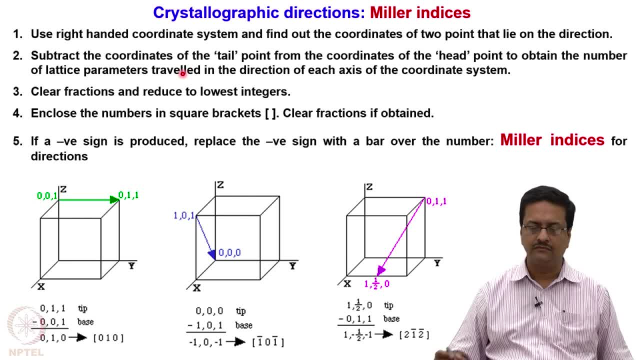 direction of each axis of the coordinate system. Then, by doing this subtraction, if you end up getting fractions, you clear the fractions and reduce it. the numbers to lowest integers, Enclose those numbers in square brackets. clear fractions if obtained, And if you have a negative sign produced, replace the negative sign. 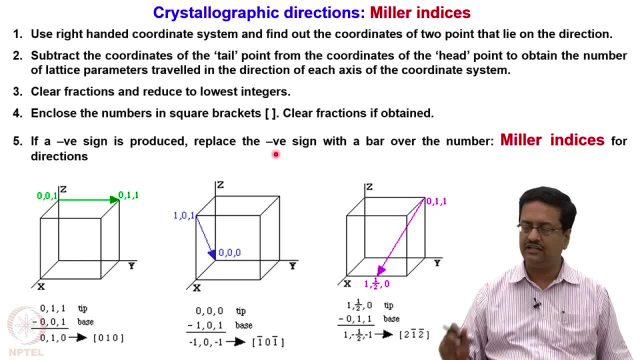 with a bar and then that number. the set of three numbers are called the Miller indices of that particular direction. So here are three examples at the bottom, the extreme left one. I want to know what is the direction from this point, which is 001 to 011.. So the tip is: 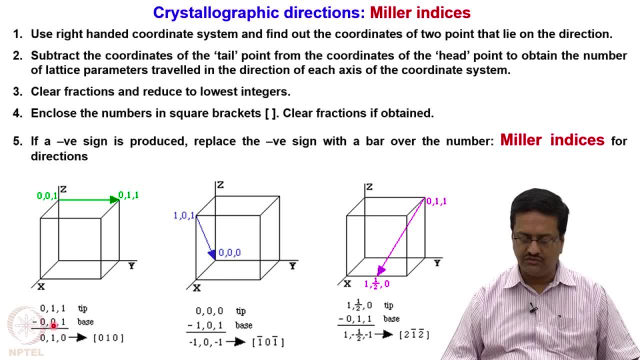 1 1, the base is 0 0 1.. So I am subtracting the base coordinates from the tip coordinates and I am getting the number 0 1 0.. So that 0 1 0 should be written in square bracket and. 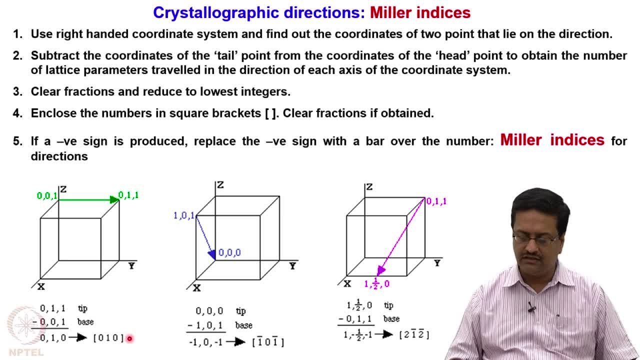 the particular direction indicated here in green is the 0, 1, 0 direction. So these are the Miller indices of that particular direction. Let us see the second one Here. the direction is from this corner which has coordinates 1, 0, 1, from there it we are trying to. 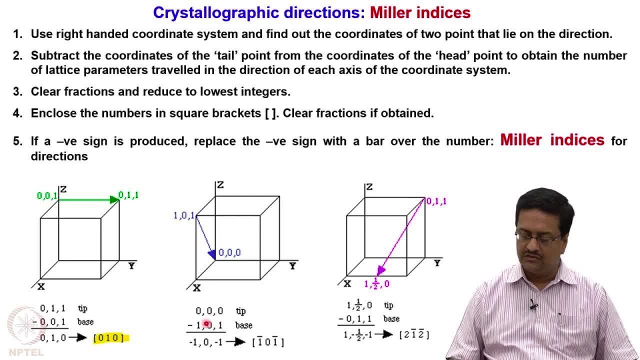 find out what is the direction towards the origin. So the origin is the tip, the base is 1 0, 1.. So what we do is we get the base. So since the base is 1 0, 1, we can write 1 0, 1.. So the base is: 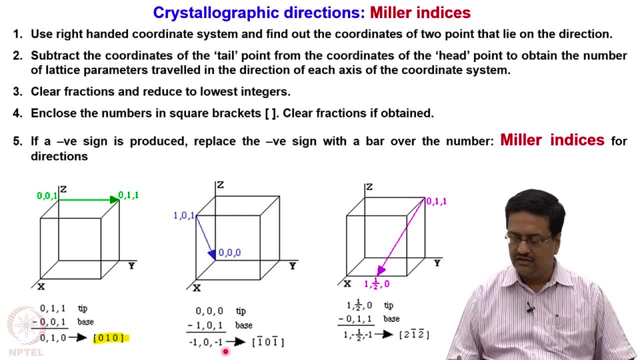 have on subtraction minus 1, 0 minus 1.. So when we represent it within third bracket or the square bracket, then the Miller indices for that direction is 1 bar, 0, 1 bar. In the same manner, in this case you have from 0, 1, 1. we are trying to find out the direction which is the middle point of this edge. 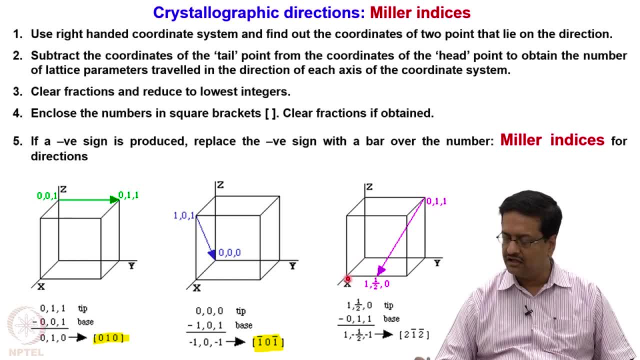 So this is 1 along x, half along y and 0 along z. So this 1 half 0 is the tip and the base is 0 1, 1.. So on subtraction it becomes 1 minus half minus 1.. 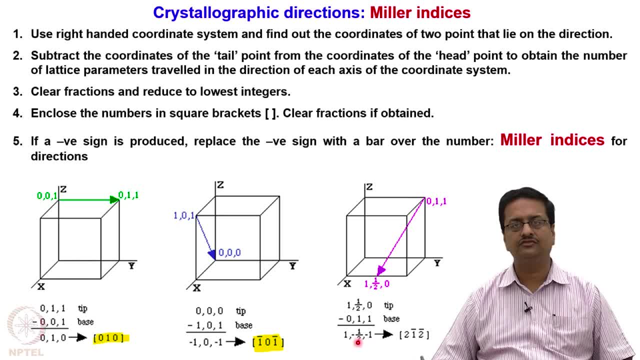 Now we have a fraction here, So this fraction has to be cleared. So we multiply this 3 numbers by 2 to remove the fraction, So it becomes 2: 1 bar, 2 bar, and that 2 1 bar, 2 bar is the Miller. 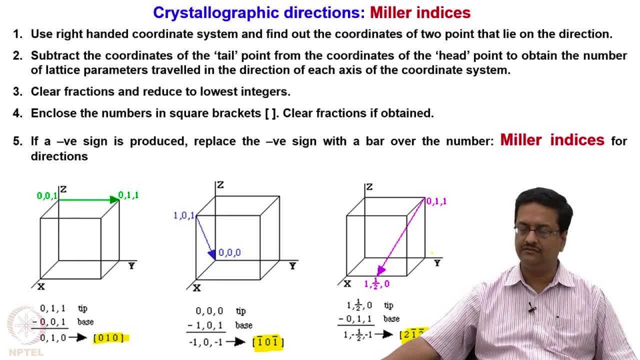 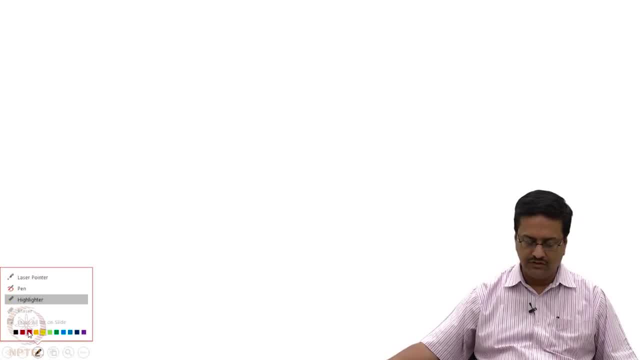 indices for that particular direction that we have seen now. Now let us do a few more, because on subtraction, this will be 1 bar, 2 bar. So here we have 3 number divided by 2.. So we are would like you to learn this and do it yourself, and we should do it from the scratch again. 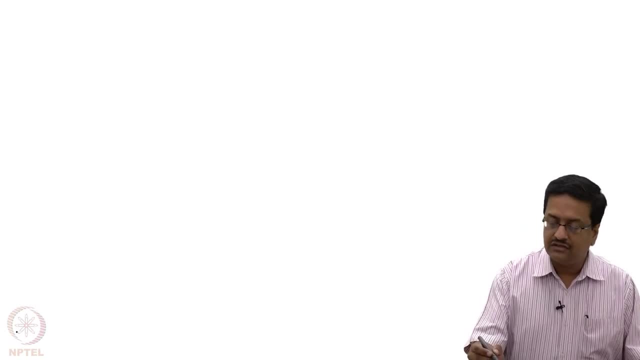 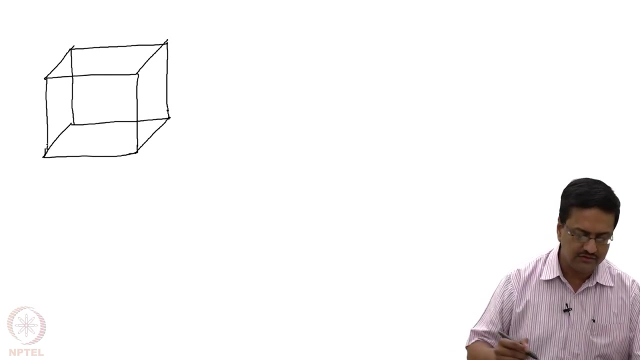 Because there are some aspects which I would like you to understand here. So I am drawing a cube and I want to know what is the direction from this corner to the other corner. So this is a body diagonal. so the starting point, origin, is 0, 0, 0. the ending point: coordinate is 1 1 1.. So the at the right point, thisyard shell is here. so this is a to the opposite corner, As I have seen the direction which I want: Intelligent centimeters straight line length, which have already represented here. 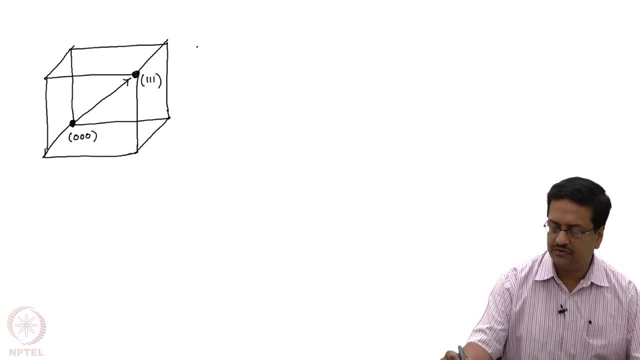 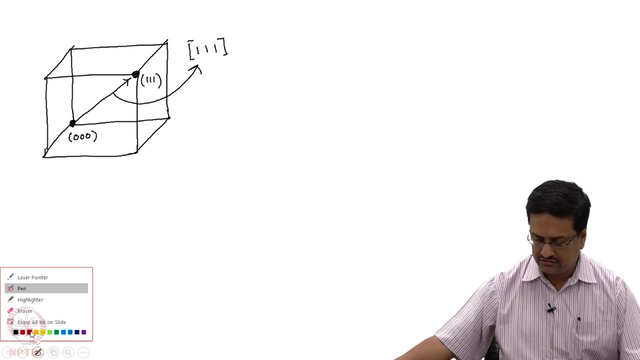 so I have to do this. So I am trying to know where all the adjourn points, the diagonals and cchar lines. if you subtract the coordinates of base from the tip, you get 1 1, 1 and hence the direction that we have got has Miller indices: 1 1, 1.. Now, if we try to see the direction from this, 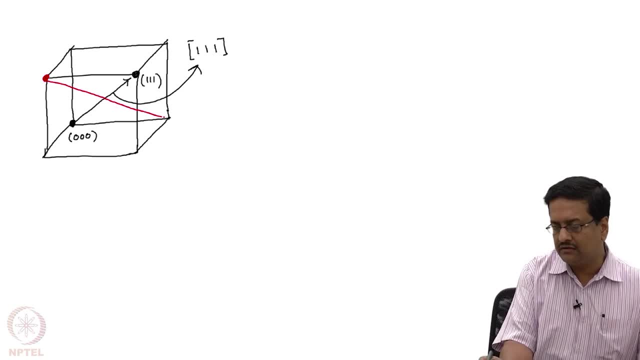 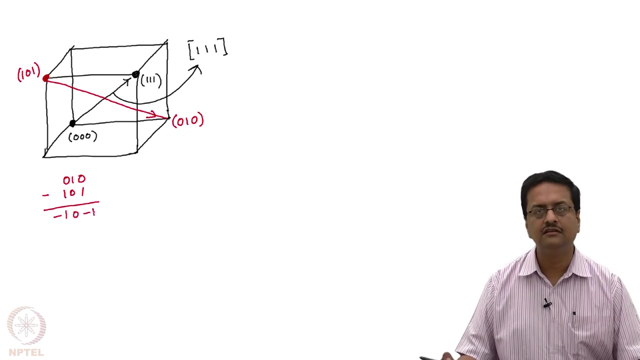 corner to the other corner of the unit cell. So what is the coordinate of this corner? it is 1 0, 1 and the tip is 0 1 0.. So if we subtract 1 0 1 from 0 1 0, what we get is minus 1, 0 minus 1.. So immediately sorry, 0 1 minus 1, I am sorry. 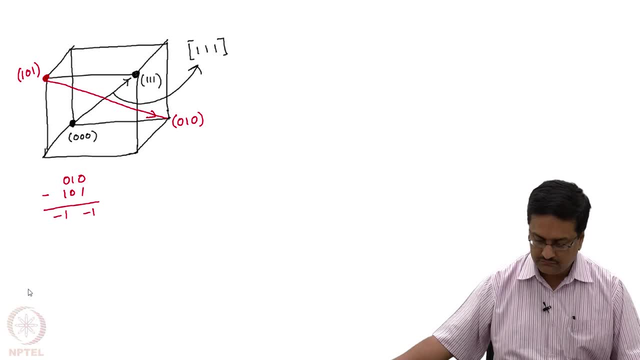 0, 1 minus 1, which means the Miller indices for that plane, that for that direction will be 1 bar, 1, 1 bar. So if we subtract the coordinates from this corner to the other corner of the unit cell, now you compare these two directions, they have same indices, 1, 1 and 1, with a different sign: minus. 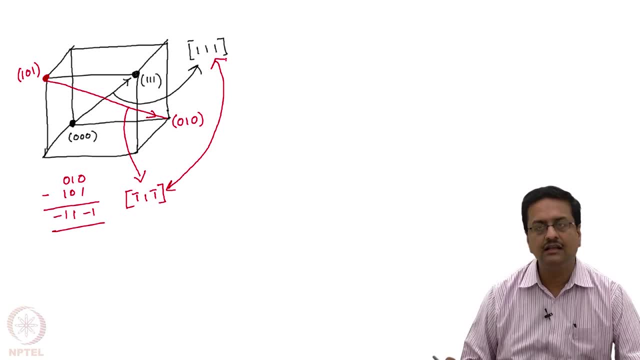 on two cases, and they are body diagonals. So these body diagonals are equivalent directions, and they are equivalent directions, and and they are can be represent as 1 1, 1. within this greater than and less than sign, it means that you are referring to all the planes which can be formed by combination of 1, 1, 1 with plus. 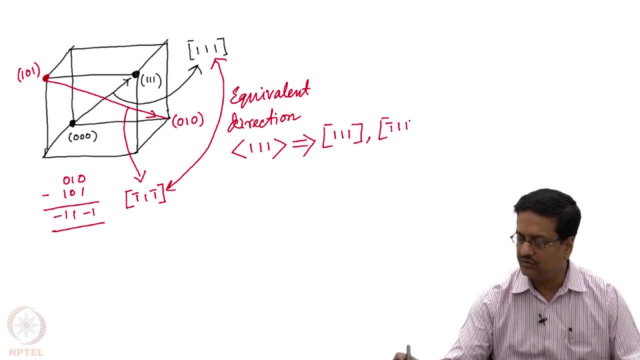 and minus signs on each, So 1 bar 1, 1, 1 bar 1 bar 1, 1, 1 bar 1, and so on. all possible combinations would represent one or the other body diagonal having different directions, and they are called. 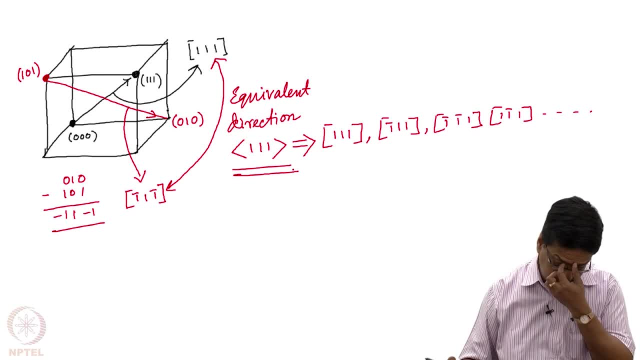 the equivalent directions. The next one that we would like to draw here, a direction with fractional coordinates in it. So we start from a point which is half 0, 0, and we go to another point here which is 0, half 1.. So 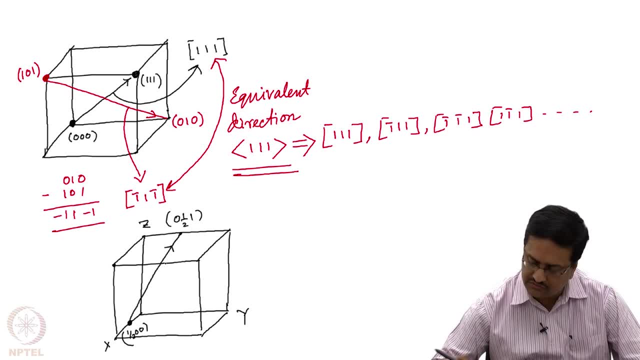 we are trying to find out the Miller indices of that particular direction. So we should do this: 0 half 1 is the tip and half 0, 1 is the base. So we should subtract the base from the tip So we get the base of this. congruent results is 0 half 1, which is 1, and the ray of shift back does: 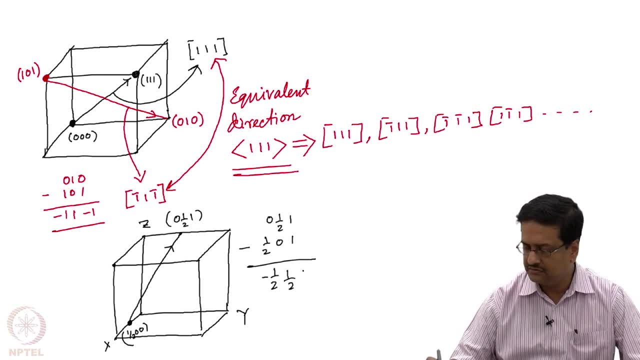 not affect this 5.. So we should give this 0 half 1, which is 0 half 0, minus half half. sorry, the base is 0 minus half 0, 1.. So now we have two fractions. So 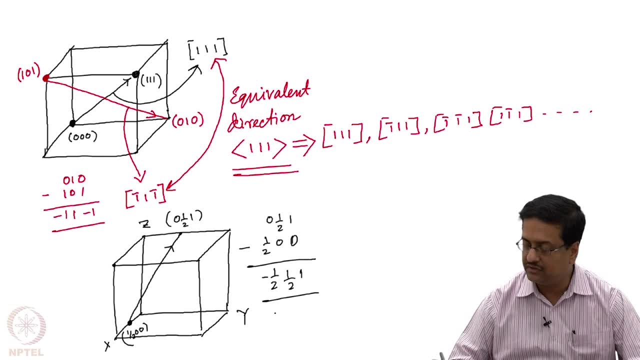 we need to clear the fractions. by multiplying by 2, we convert it to minus 1, 1, 2.. So the corresponding Miller index indices for that particular direction is going to be 1 bar 1, 2.. So this is how one should generate the Miller indices of the directions. 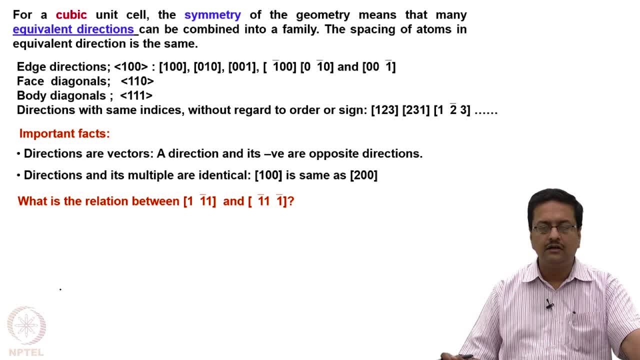 So for a cubic unit cell, the symmetry of the geometry means that many equivalent directions can be combined into a family. as we have Indicated, the spacing of atoms in those equivalent directions is the same. So when we say edge direction, we are talking about the directions 1, 0, 0, 0, 1, 0, 0, 0, 1 and all. 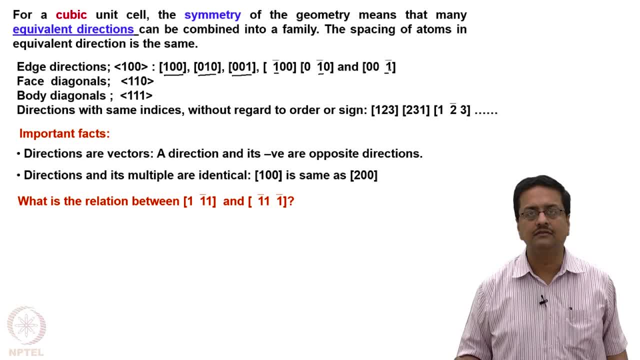 combinations with negative signs of 1.. These are the directions along the edge. The phase diagonals will mean they are of the family 1- 1- 0 and the body diagonals are of the family 1- 1- 1. that we already have seen. And directions with same indices, without regard to the order or sign. 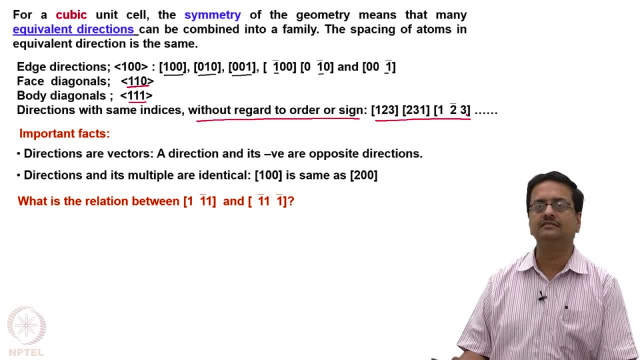 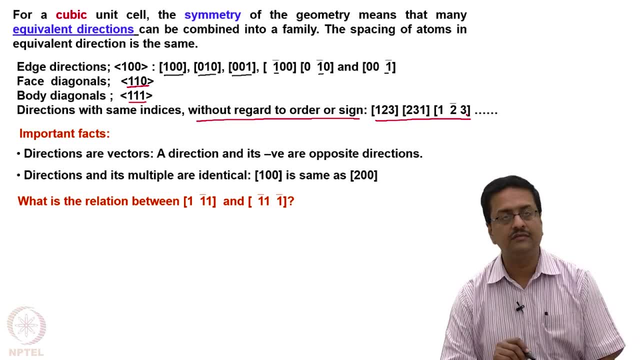 are also can be classified as equivalent directions. What are these directions? So two things to be remembered. Directions are vectors, So a direction and its negative are opposite directions. That means, if we write 1, 1, 1 and if we write 1 bar, 1 bar, 1 bar, that 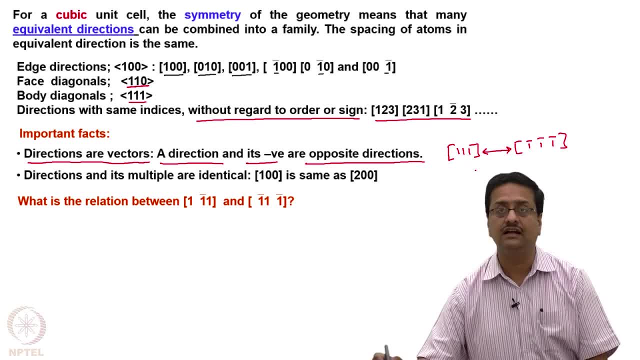 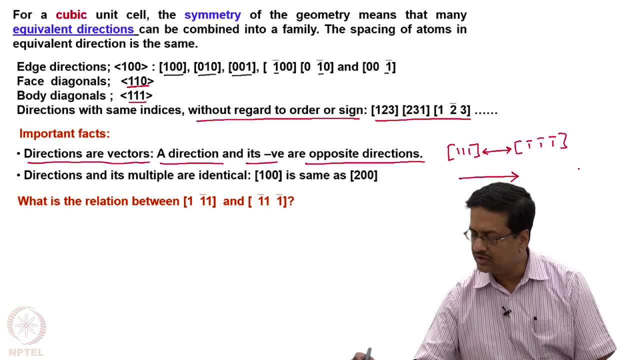 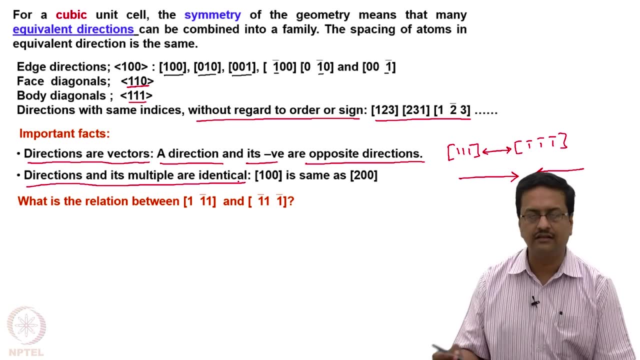 means these two are opposite directions. If 1 1- 1 mean a direction left to right, a direction 1 bar, 1 bar, 1 bar would mean right to left Directions and its multiples are identical. That means 1 0 0 is same as 2 0 0.. So in case of directions, one should always reduce the HKL. 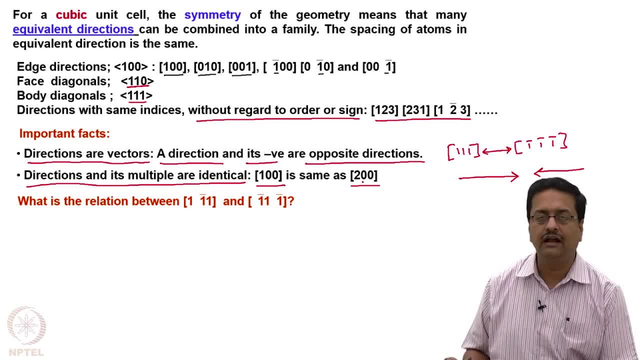 indices to their minimum value and write that as a the correct Miller indices for those directions. So what is the relation between these two? point, two directions: 1, 1 bar 1 and 1 bar 1, 1 bar. The answer is antiparallel or opposite directions, because here the one which was plus is now minus. 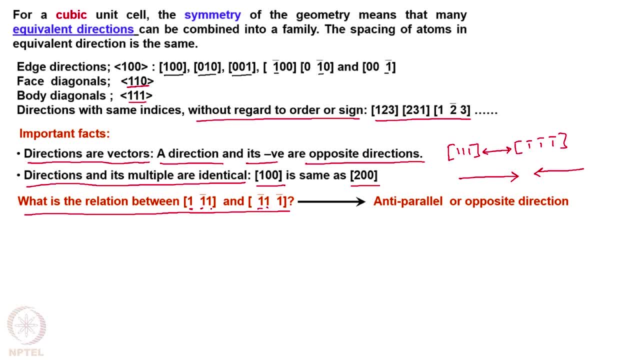 The one which was minus is now plus, and the one again which was plus is now minus. So in the same manner as we saw, 1, 1, 1 and 1 bar, 1 bar, 1 bar- Our opposite direction, it applies for other combinations also. 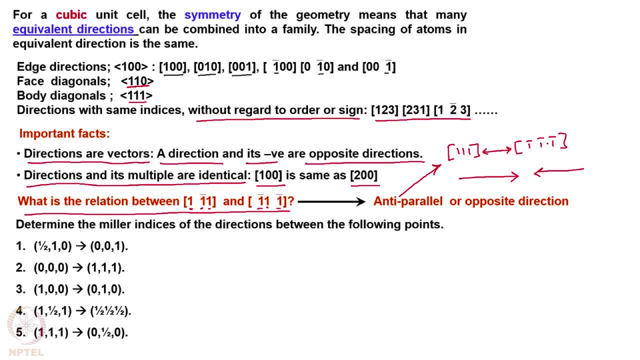 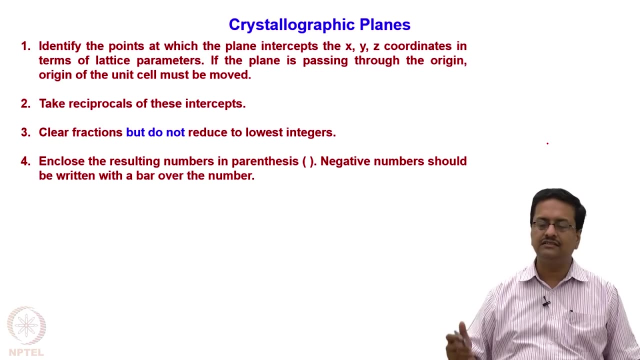 So I would like you to practice at home that determine the Miller indices for the direction between the following points. There are five such examples I would like you to do yourself. Now I would like to move to the crystallographic planes. We would like to designate the planes. 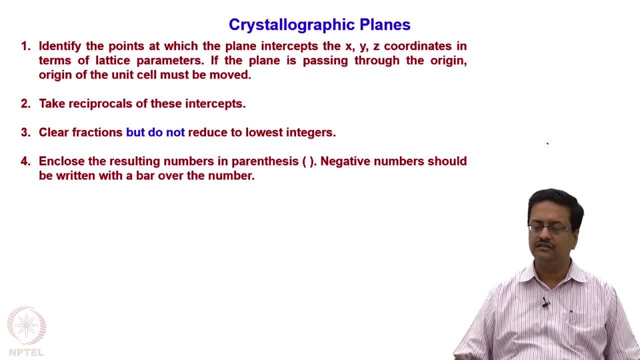 in the same manner as the directions, using three indices: H, K and L, and we try to determine those Miller indices by using a procedure which I am going to describe now. So what we need to do is we have to identify the plane in the lattice. We need to find out. 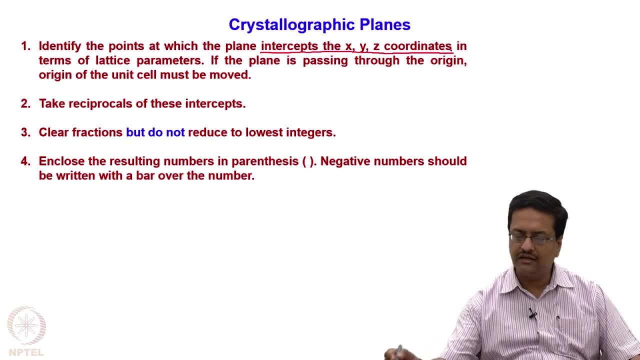 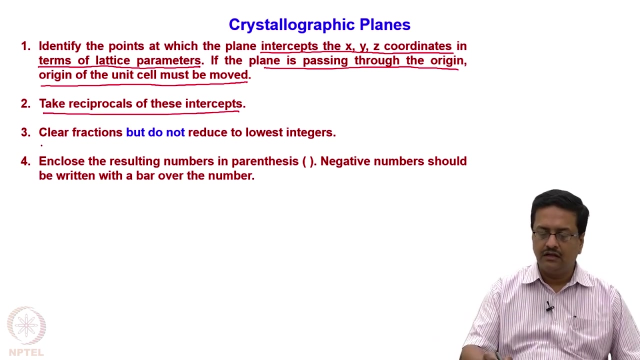 the intercept of x, y, z coordinates. in terms of lattice parameters, the plane is passing through the origin. the origin of the unit cell must be moved to a suitable position, such that the origin does not coincide with the plane anymore. then one should take the reciprocal of these intercepts. clear the fractions, but do not, do not reduce to lowest. 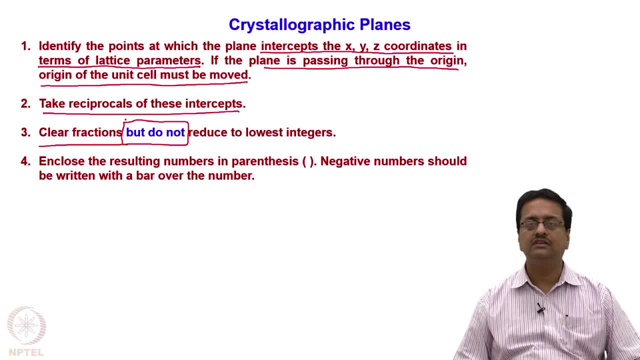 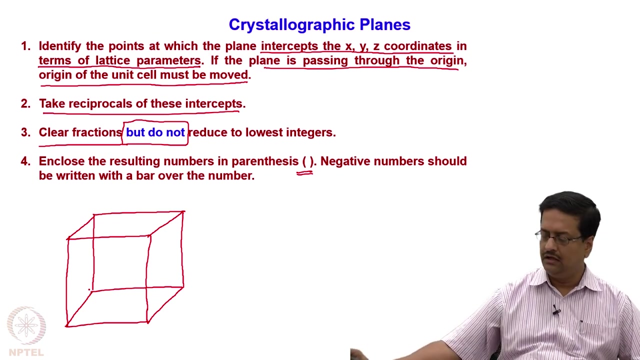 integer, which is different from what we saw in case of directions, And then enclose the resulting numbers in first bracket, and negative numbers, as usual, should be written with a bar. So let us see the case of a few examples. So I have drawn a cube and in that, as usual, this is my x direction, this is y and that. 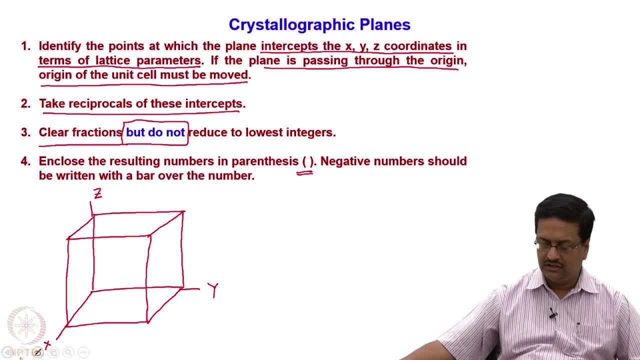 one is my y direction. So we have shown one equilibrium. there is another equilibrium is z. here I want to designate a plane which is like that: this is one face. So what are the intercepts of this face on x, y and z? You see, this face is parallel to both x and 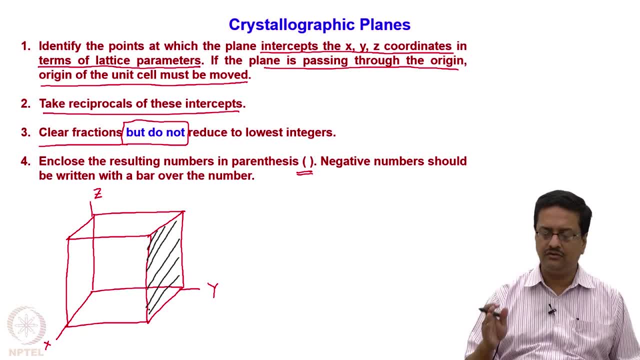 z. So this face is not going to have an intercept on x and z. that means the intercept of this plane with x and z are infinity and this plane meets the y axis from the origin at a distance 1.. So these are the intercepts. 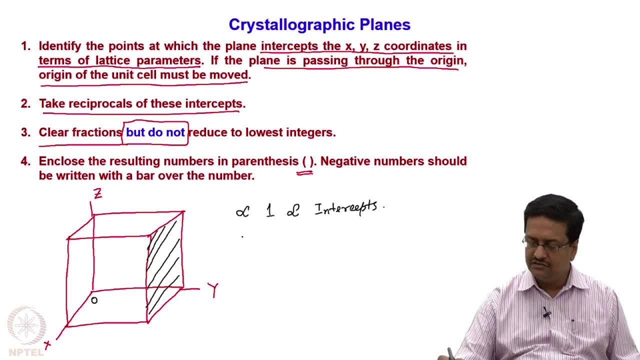 So if I take reciprocal of these intercepts, I end up getting 0, 1, 0.. There is no fraction to be cleared, there is no nothing to be reduced or anything. So the Miller indices for that plane is 0, 1, 0.. 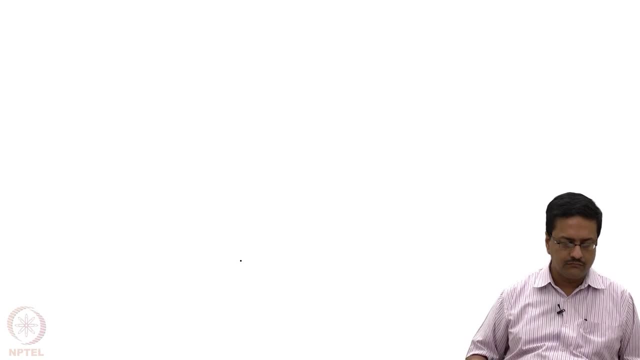 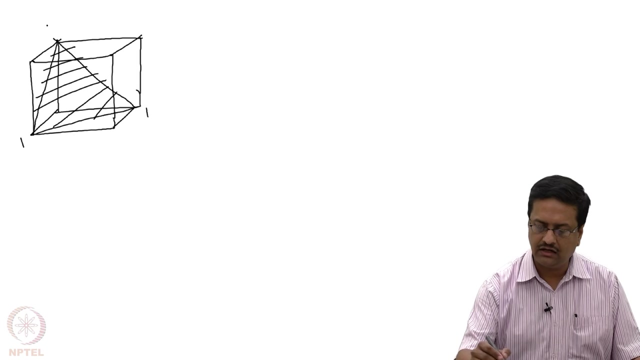 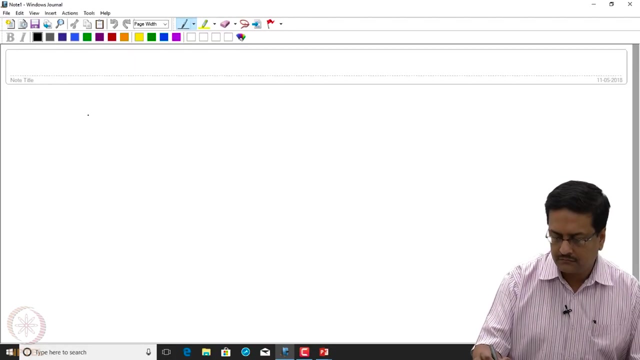 Now let us see a different plane, the plane which is here. So the intercepts are 1, 1 and 1, the reciprocal is again 1, 1, 1.. So the plane is simply 1, 1, 1.. Let me draw a few cubes. 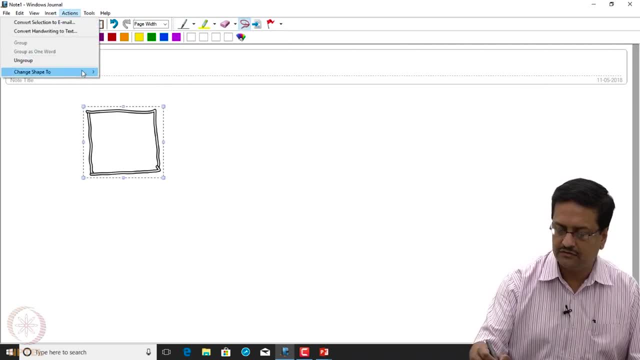 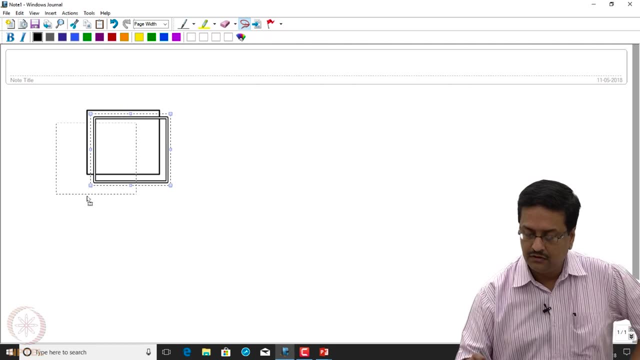 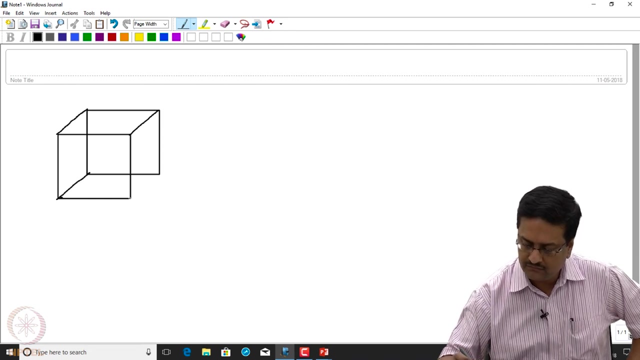 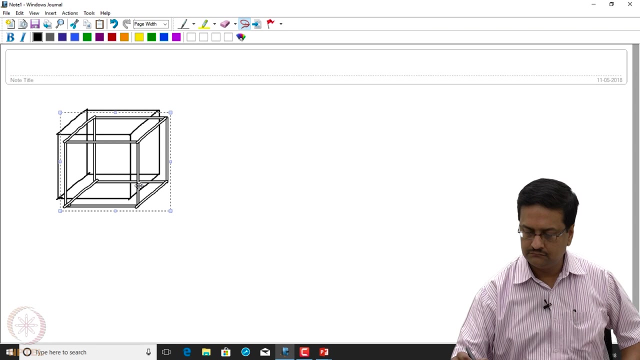 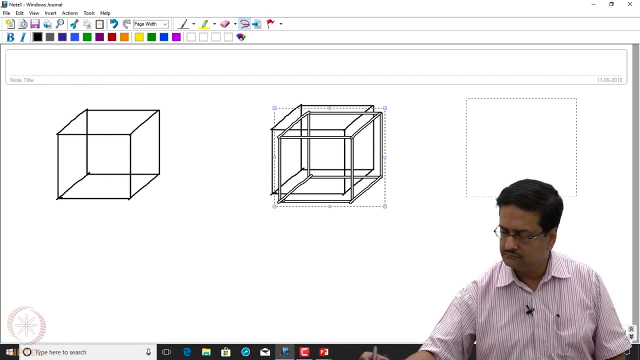 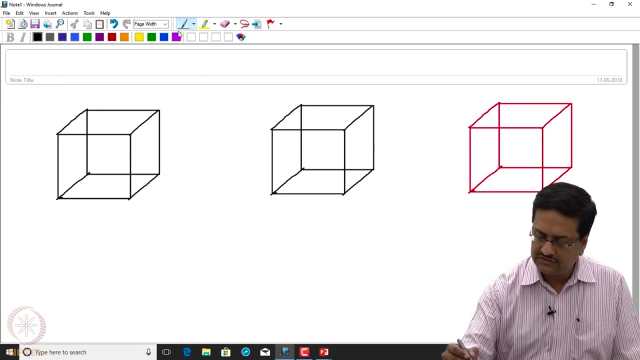 Here so that we can continue drawing the Miller indices for a few set of different planes. We have seen that the plane which is here is designated as 0,, 1,, 0, what should be the designation of that particular plane. You see that this particular plane is passing through the origin. 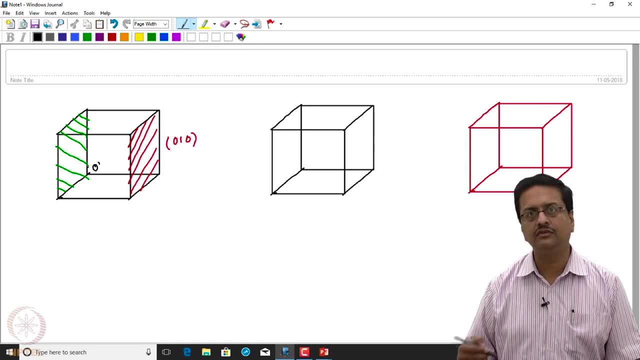 So we need to shift the origin to a suitable location, such that the origin is no longer on the plane. So instead of having x, y, z like that, I would shift this origin here so that this direction is plus x, plus y. 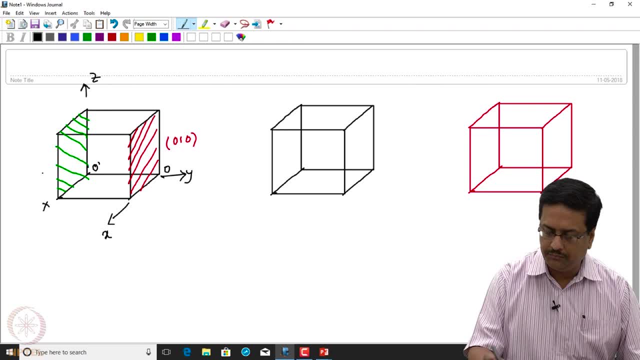 This direction is plus x, the backward direction is minus y, and so on. So now, with respect to this new origin, this plane is parallel to x, parallel to z and has y intercept minus 1. So the intercepts are minus. 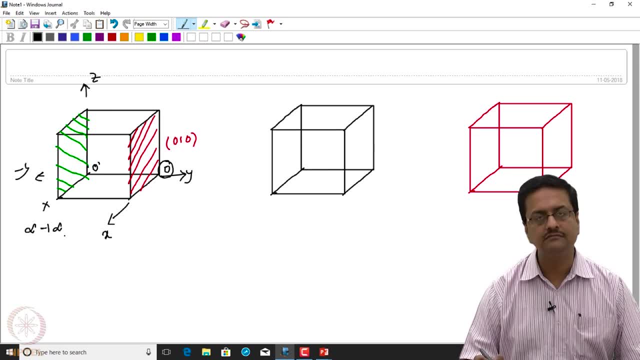 infinity minus 1 infinity. So on taking reciprocal it becomes 0 minus 1, 0.. So the Miller indices of that particular plane is 0 minus 1, 0.. What do we see? These two planes are parallel. they have the indices same, but the sign opposite. Now let us see a situation where 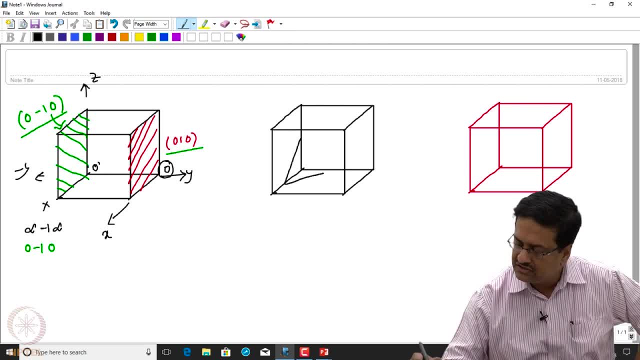 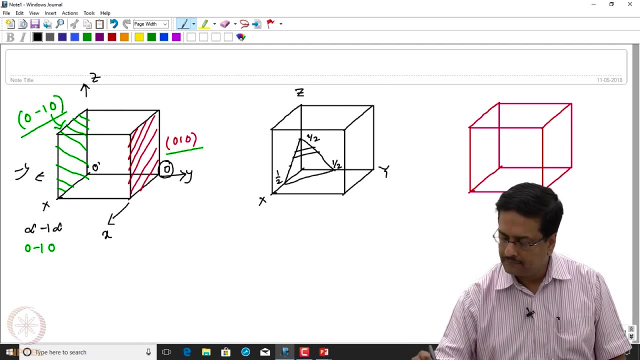 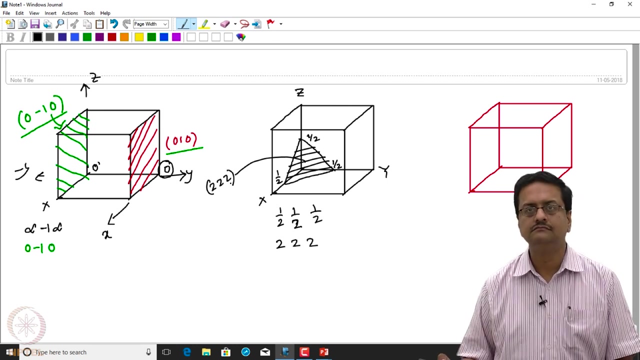 we are trying to draw a plane which intercepts at half on both all the three, x, y and z. So the intercepts are half, half half. So the reciprocals are 2, 2, 2, nothing too clear. So that particular plane should be designated as 2, 2, 2 plane. Now, if you remember the plane, 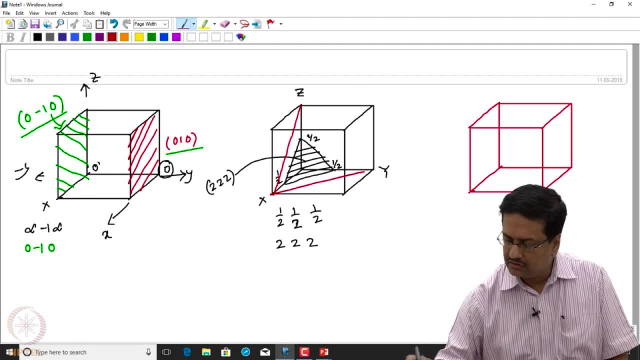 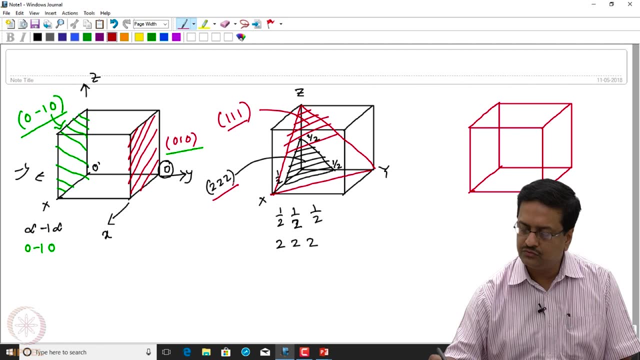 which was like this: Combine connecting the three diagonals, 3, 3 corners. that plane we designated as 1, 1, 1.. You see now the 1, 1, 1 and 2, 2, 2 are set of parallel planes and but they are different. 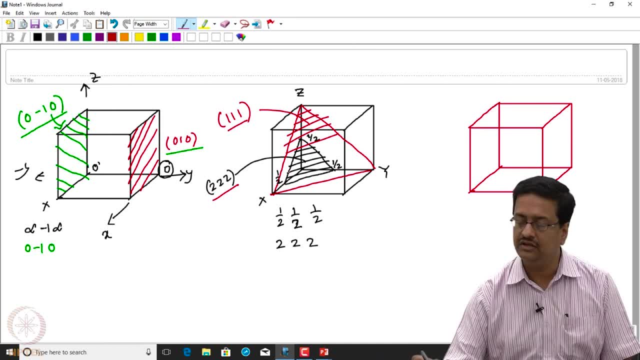 The plane 2, 2, 2 covers a smaller area inside the unit cell compared to the area covered by 1, 1, 1 plane. Now let us say that I am placing one here and 2, 1, 1 and 2, 1. they areijше ng so this. 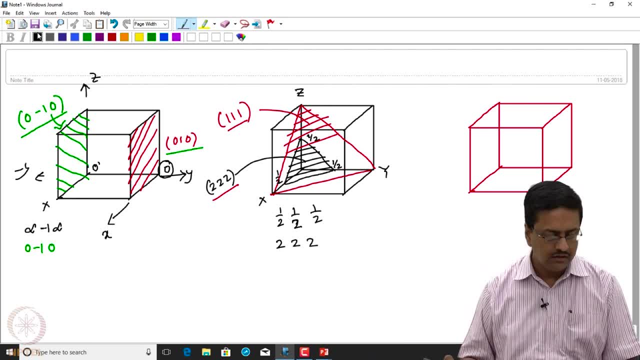 here I can get a fewader threes突 with other distribute interaction. that was free at half fire, 0 minus 1.. Now on taking this one particular plane with a point. the intercept here is chief. So now on the third box. here I would like to draw a plane like this, the intercept here: 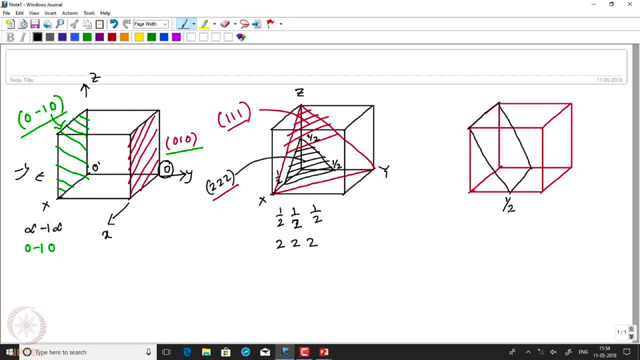 is half. So that means along x, y and z. we have this plane which is parallel to x, y and z point. Therefore, I draw a plane with a straight line, y, which will be same here, along which of course I will мин the second. We draw a plane like this because colouring is same, but 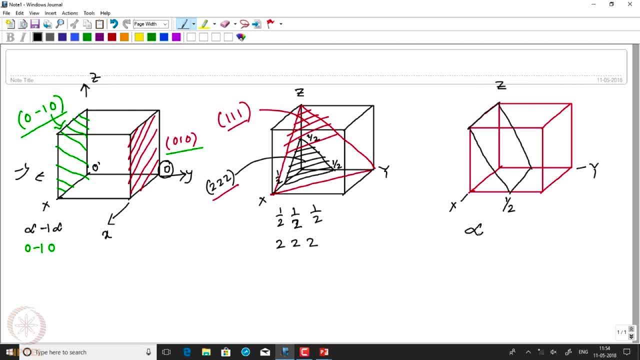 parallel to x axis. that means x intercept is infinity along y. it has intercept half along z. it meets z at 1 unit away from the origin. so z is 1.. So now take reciprocal: set becomes 0,, 2, 1, which means the Miller indices, for that would be nothing but 0,, 2, 1.. 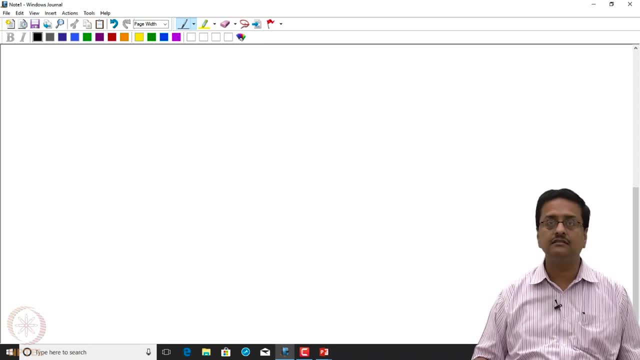 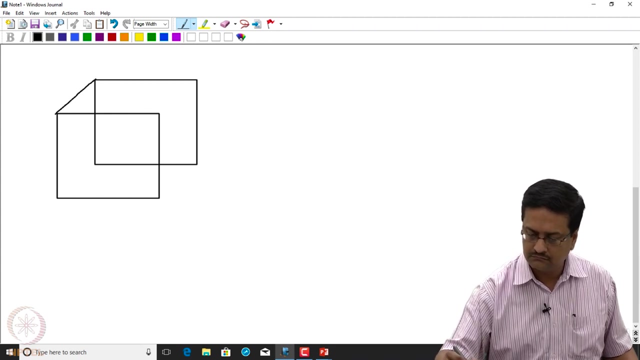 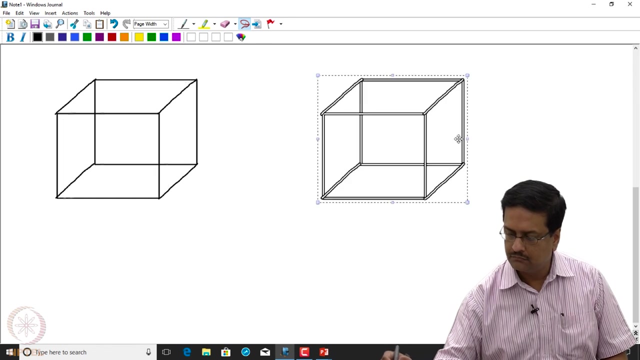 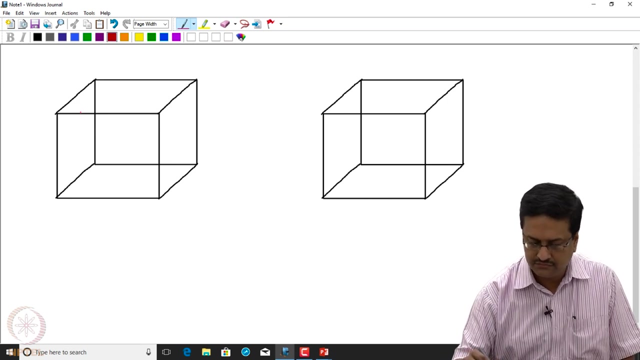 Now let us see a different situation. Suppose we want to identify the Miller indices of this particular plane, this has intercept one-third with respect to that origin. This intercept here is half and here this intercept is three-fourth. So now with respect to the origin, location z, this set is half. so zman to z set is half. So now we can now write the problems of x persons, of Momin, seichelink, V, Q, perform the same product, hb to the origin, to form a single максимum manif suggestion to the origin. Here again it empowers the elements and the, που has to be tripled like that, because on the 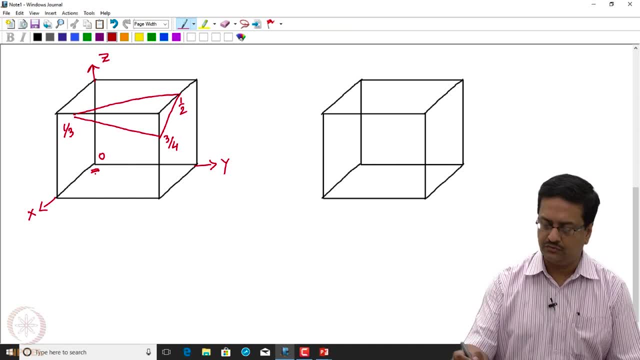 here. it is difficult to find out where this plane would go and meet x, y and z, and also this origin is not set sitting on this particular plane. but still we can move the origin to a suitable position such that we can easily determine the intercepts. So what we will do is we move this. 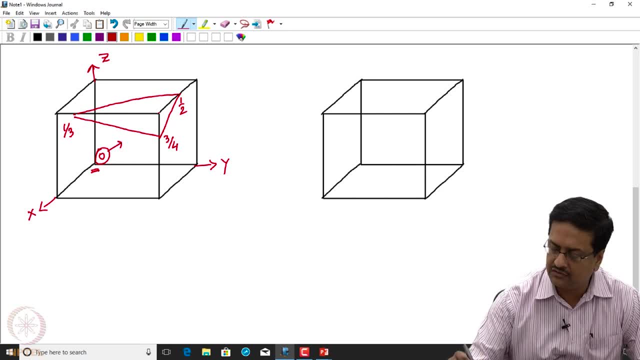 origin from here to the other body, diagonal point, which is here, and we write it as a new origin. So, with respect to that, this is the plus x, this is the plus y, anything above is plus z and anything below is minus z. So now, with respect to this new origin, 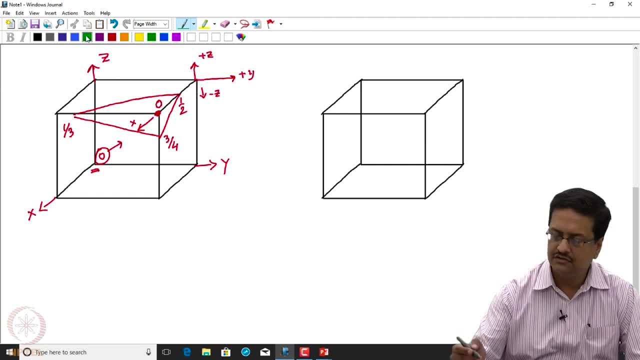 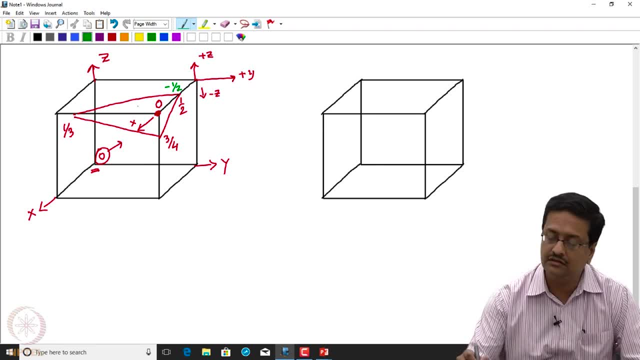 from that origin. now this origin, this becomes minus two third and the z intercept, which was three fourths. respect to dot origin means it is measured from the bottom most position here to that point there. So this was three-fourth. that means now it has become one-fourth, with a negative sign because 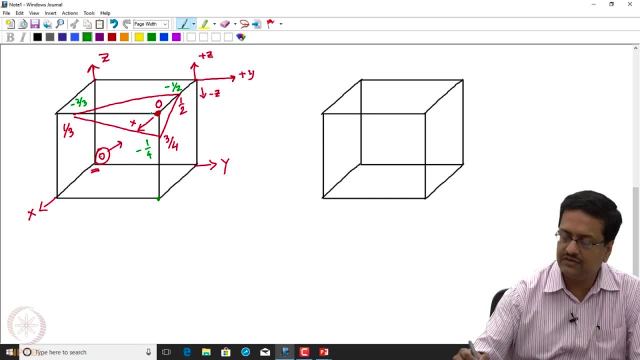 it is downwards. So the new intercepts with the new origin are minus half, minus two-third and minus one-fourth. So now we would like to clear the fractions. so when we try to clear the fractions, no, first we need to do take the reciprocals. So when we take the reciprocal, 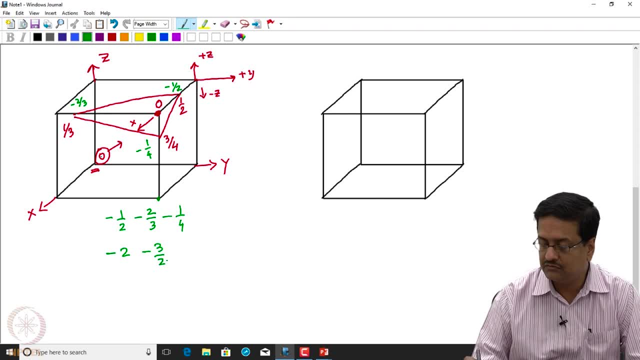 it becomes 2 minus 3 by 2 and 4.. So now we need to clear the fractions. So when we try to clear the fractions we multiply by 2. So it is minus 4, minus 3, minus 8.. So the Miller indices for that particular plane becomes: 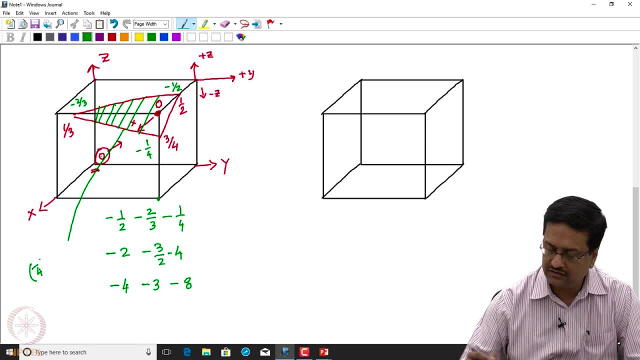 4 bar, 3 bar, 8 bar. Now I would like to give a homework for you to do and come back in the next class and we will see how this can be solved. So, in this particular cube that I have drawn here, 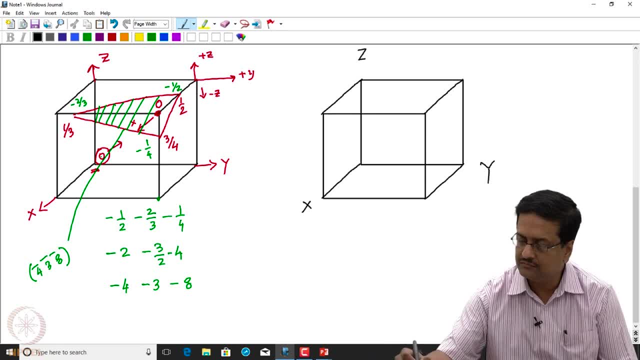 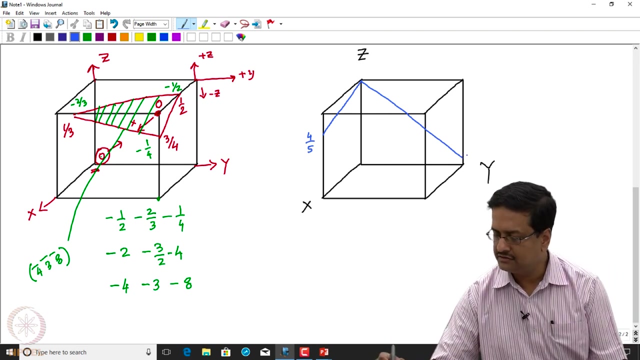 x, y and z. as usual, I am drawing a plane which is having an intercept on z-axis here as 4 by 5, and it has again an intercept on z-axis at 1 by 6.. And this is the plane. What would be the Miller indices for that plane is an assignment for you.